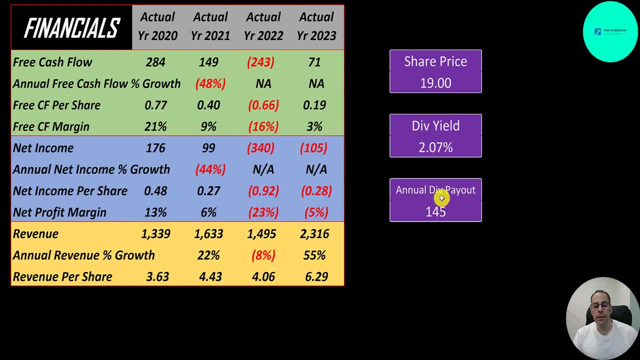 It does make it hard to value. Their dividend yield is 2%, which means they pay out $145 million in dividends for the year. Their free cash flow is half of that, so something to give. They need to generate more free cash flow or cut their dividend. In 2020, they generated a. 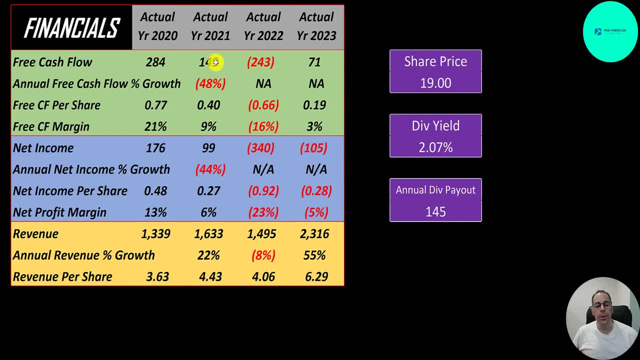 good amount of free cash flow, more than enough to cover their dividend. 2021 was almost identical to the dividend. Net income is the profit or loss on the income statements, revenue minus expenses. That's positive in 2020 and 2021, negative in 2022 and 2023.. Revenue is a sales for the company. 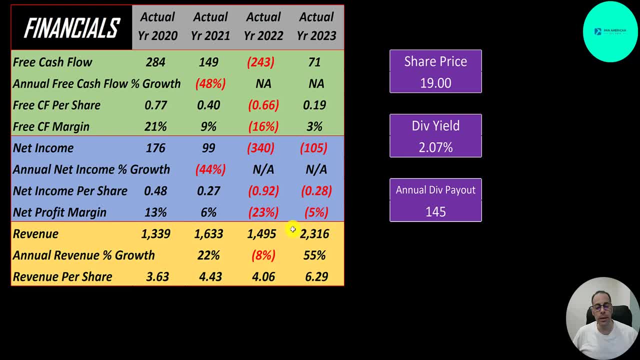 and that goes up from $1.3 billion to $2.3 billion. It dipped a little from $21 to $22 to $28, but up 55% into 2023.. Their revenue per share is $629.. One share price is $19,. 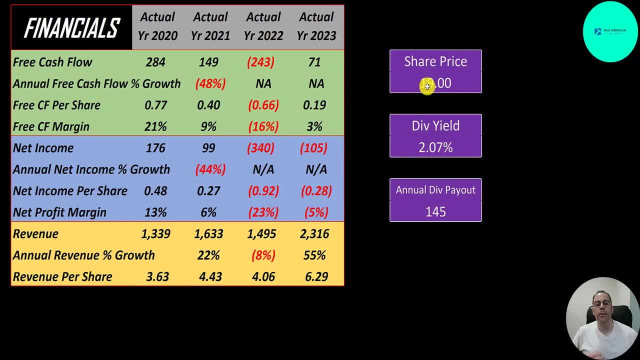 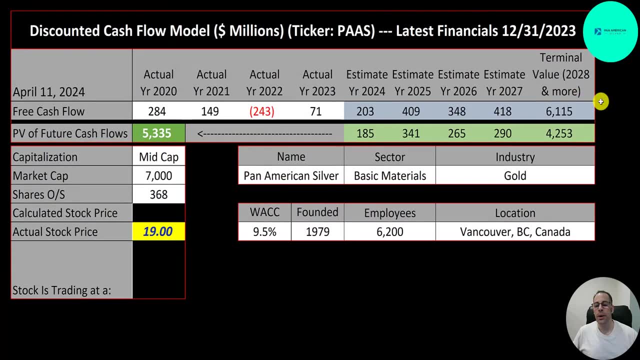 so your piece of the company is $629, but the free cash flow generated per share is only $0.19.. We estimated four years of future free cash flows. We also estimated the terminal value, which is low cash flows, past year. four, that's $6 billion. We discounted those numbers back to 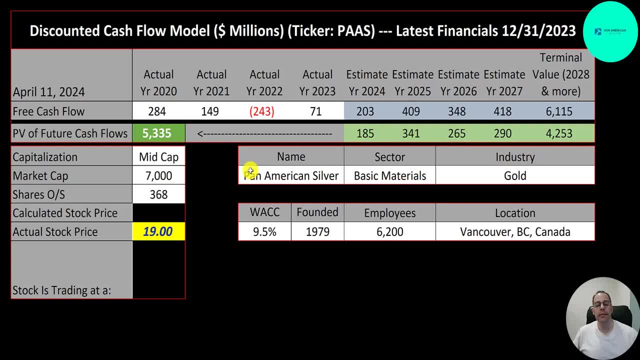 today, using the weighted average cost of capital. Here's the whack: 9.5%, We get a value in the company of $5.3 billion. We divide that by 368 million shares And we get a calculated stock price of $14, and trading at $19.. They're trading. 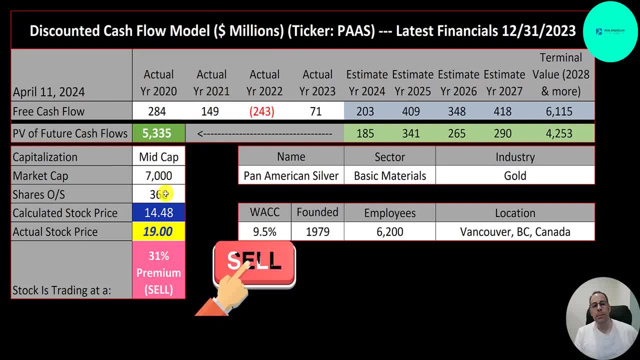 at a 31% premium. It's a sell. according to the model, The stock price is highly dependent on the price of silver and the price of gold. They're actually in the industry of gold, not silver. There's only like three companies in the industry of silver. 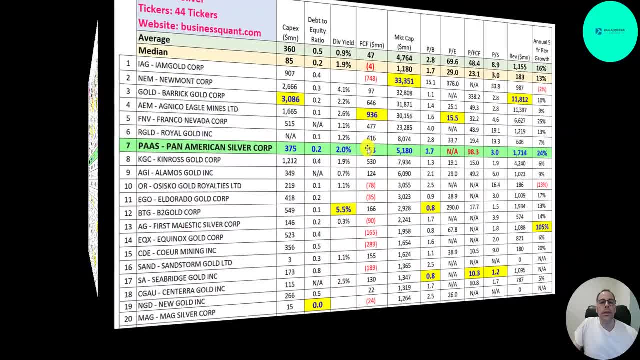 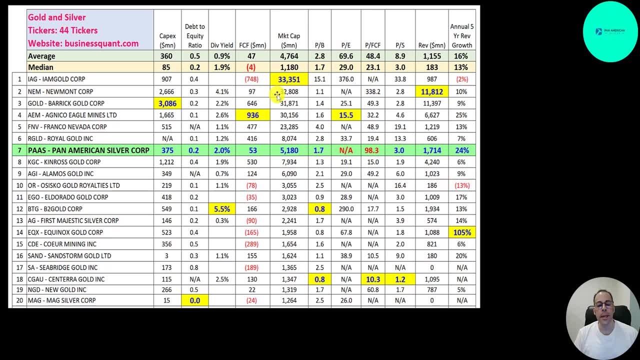 I guess if you sell any gold you're in the gold industry. There are 44 companies in the gold or silver industry And if Pan American has a number in red, they're worse than the median. If they have a number in blue, they're better. They spent 375 million in CapEx- About the average. 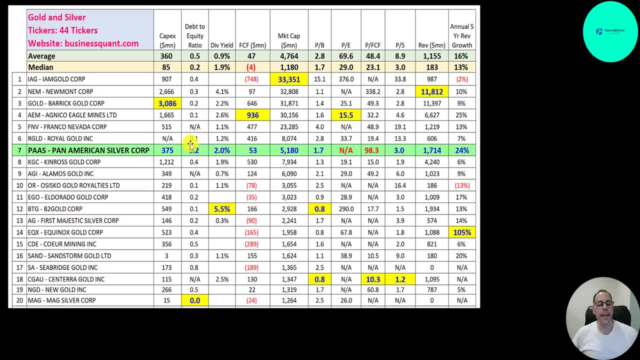 Barrick Gold spends the most: 3.1 billion. A good debt to equity ratio: 0.2.. For every dollar of equity they have 20 cents of debt. They pay a 2% dividend. B2 Gold is number one at 5.5%. 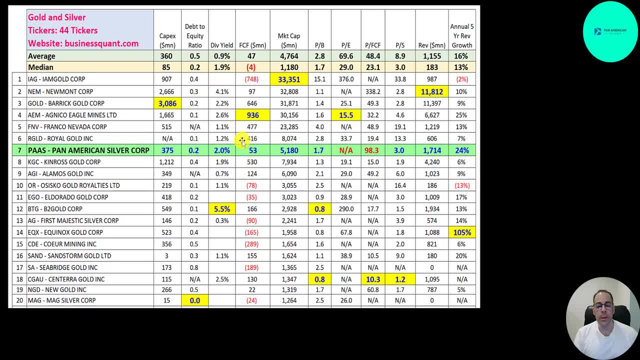 Then Newmont, 4.1%. They don't generate much free cash flow, but it's positive. It's better than the average. Agnico is number one at 930 million. They rank ninth in market cap. They should be ninth on this list. I'm not sure why they're seventh. Their price to book is equal to. 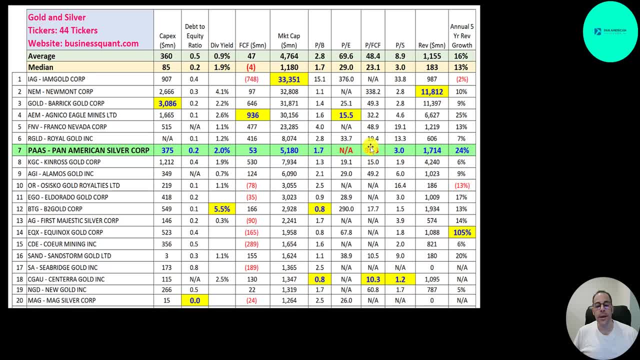 the median. We can't look at their PE. They have negative earnings. They trade at nearly 100 times free cash flow, which is not a good multiple. Three times revenue, which is good. That's equal to the median. a lot better than the average. A lot better than IM Gold. A little worse than. 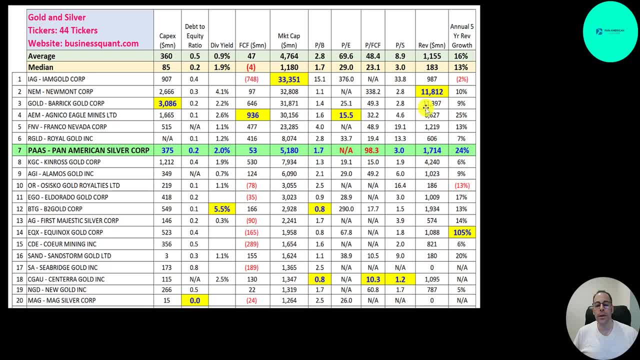 Newmont and Barrick. They generate 1.6%, 7 billion of revenue, A lot more than the median average, A lot more than number one in the industry, Triple number six, And their revenue is growing quite a bit, Their five-year annual. 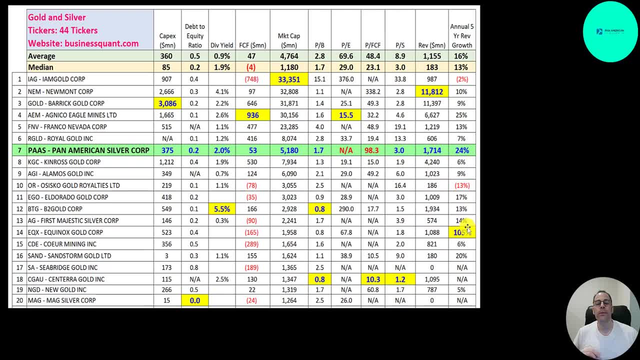 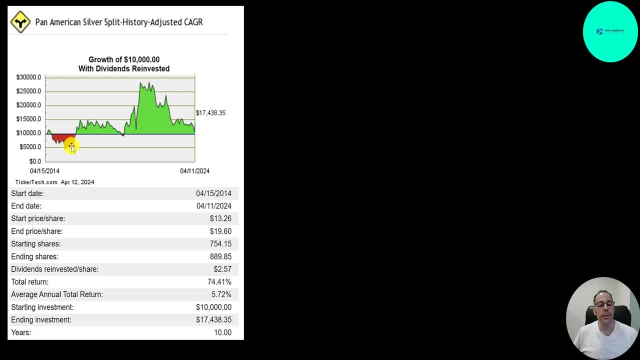 revenue growth rate is 24%. Look at Equinox: 105%. If you put $10,000 into this company 10 years ago, after a year you would have been down 50% And you probably would have sold and been pissed off. 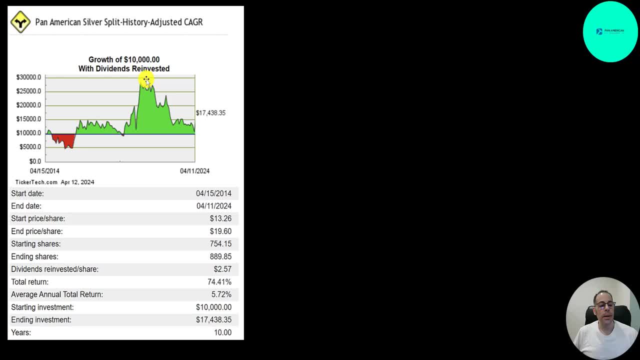 But if you still hold on, your 10,000 would have been over 25,000 in a period of time. You would have been up about 2021, seven years after your initial investment, But it has come down a lot since then. You would be up up 74% from your $10,000 investment. It would be 17,400,. 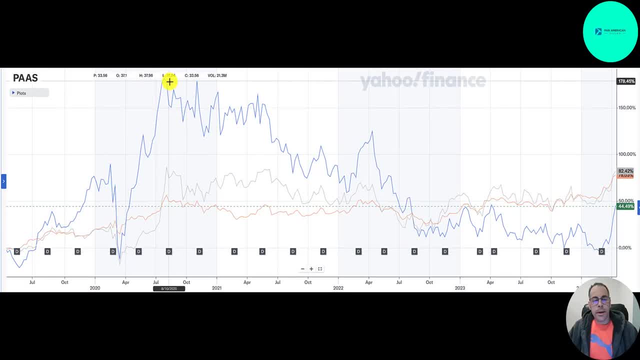 which isn't terrible. This blue line is Pan American stock price the last five years And the stock is up 45%. This grayish line is the price of silver, which is up 82%, And then gold, the orange line, up 78%, But Pan American. 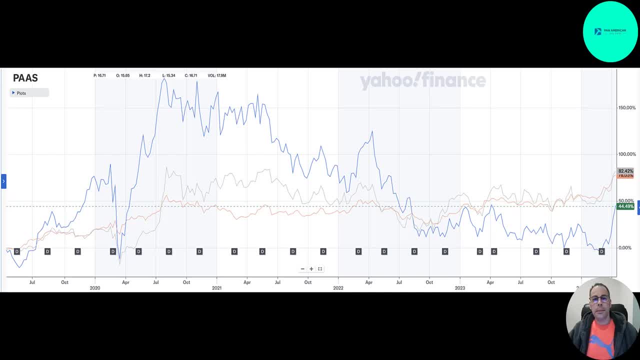 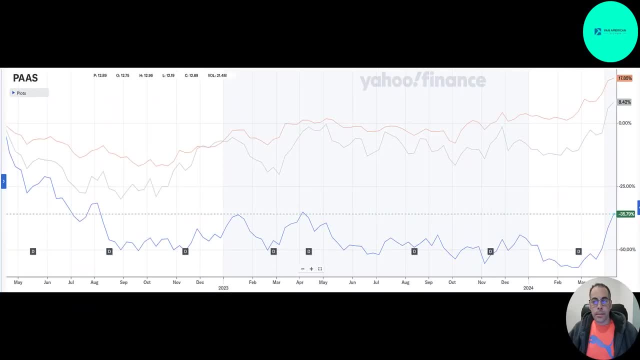 it pays a dividend. So if you add that in, it's probably close to 60%, not 44%. Still, it's trailing gold and silver In the past two years. gold and silver are up 8% and 18%. But 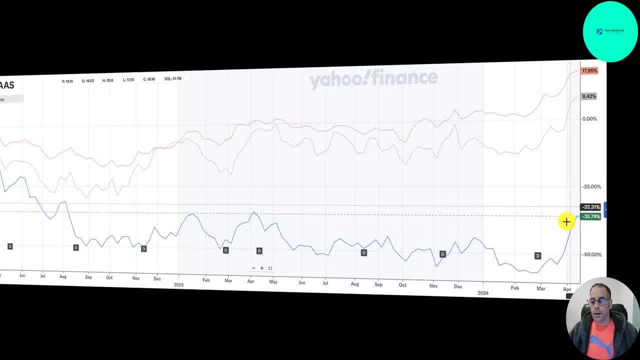 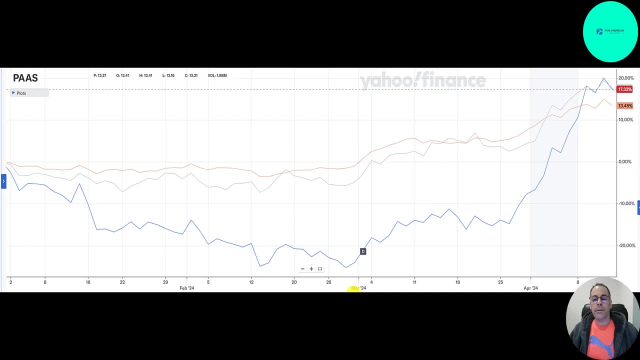 this stock is down 36%. This stock is the blue line. In the past year. this stock is flat. Silver up 9%, gold up 16%. Year to date. silver and Pan American are both up 17%. gold 13%, But in the past. three months this stock is up 24%, which beats gold and silver. So if you add that in, you're going to see that gold and silver are both up 18%. So if you add that in, you're going to see that. 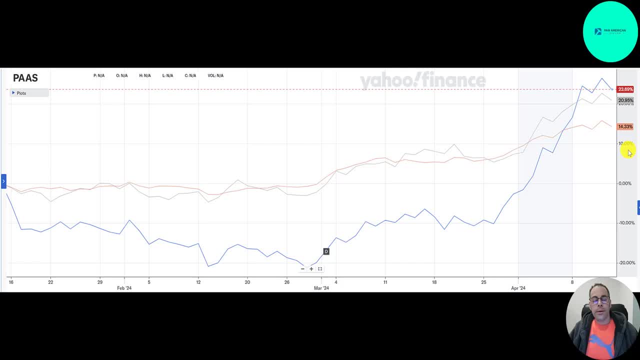 gold and silver are both up 18%. So if you add that in, you're going to see that gold and silver are both up 18%. So they don't track each other that well. There is some correlation, but not as much as I thought it. 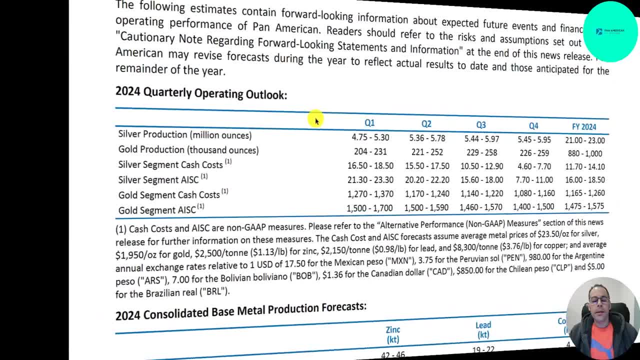 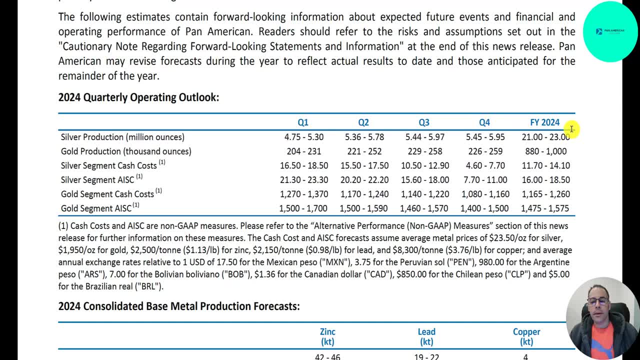 would be. Let's take a look at their fourth quarter report. Here's their outlook for 2024.. They plan to produce between 21 million and 23 million ounces of silver for all of 2024.. About 5 million in the first quarter, 5.5 million in the second quarter. about 5.7 million in the third. 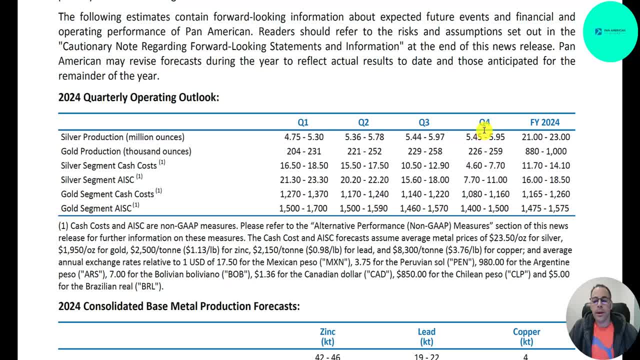 quarter and also about 5.7 million in the fourth quarter. Gold production 880,000 to 1 million ounces And they estimate the cost of silver to be between 1170 and 1410.. The all-in cost between 16 and 1850.. Gold cash cost 1165 to 1260 an ounce. The all-in cost between 1475 and 1575 an ounce. When you see AISC or all-in sustaining cost, this shows us the total cost of producing one ounce of gold or whatever commodity you're looking at. It includes all direct costs such 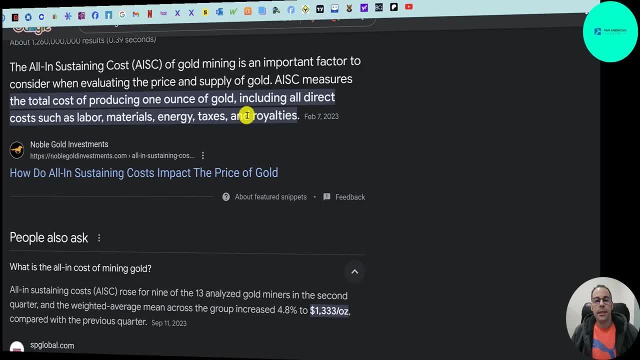 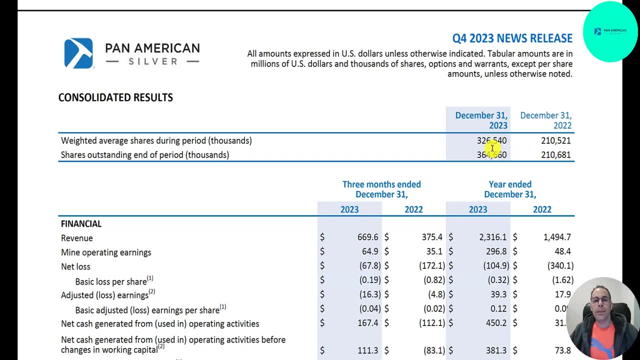 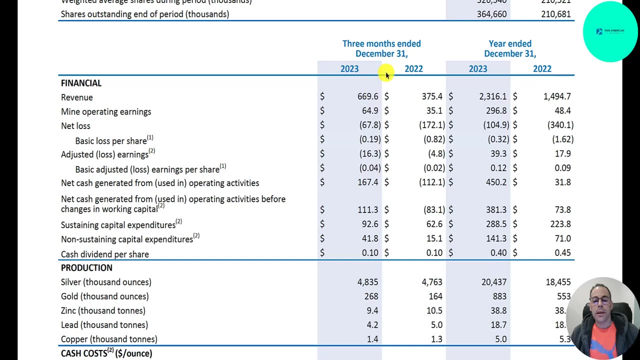 as labor materials, energy taxes, royalties. Their shares outstanding at the end of 2022 were 210 million and now it's up to 365 million. Usually, when shares increase a lot, it's due to acquisition. Fourth quarter revenue: 670 million. That's up from 375 million For all of. 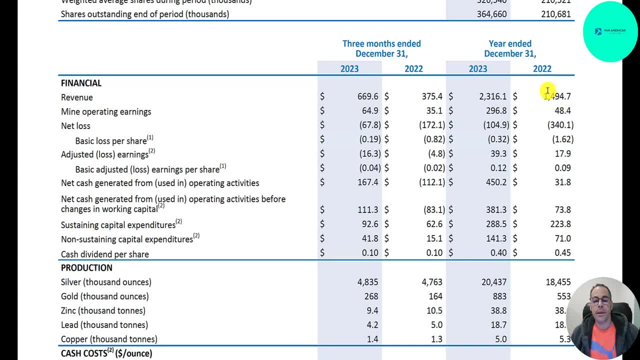 2023, 2.3 billion up from 1.5 billion Operating earnings, 300 million up from 48 million, But they still have a net loss of 100 million, which is better than last year, of 340 million. In 2023, they produced 20.4 million. 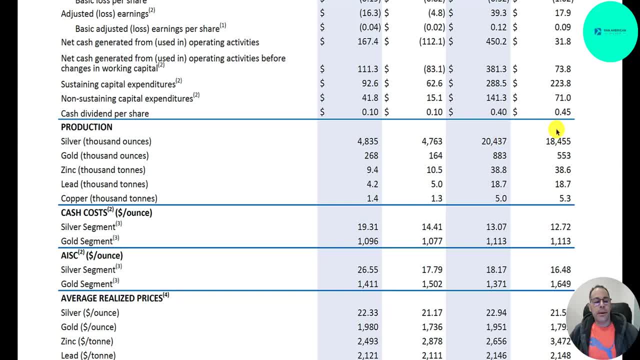 ounces of silver. That's up from 18.5 million ounces. Gold: improved 550,000 ounces in 2022, 880,000 ounces in 2023.. Zinc, lead and copper: pretty much flat from 2022 to 2023.. 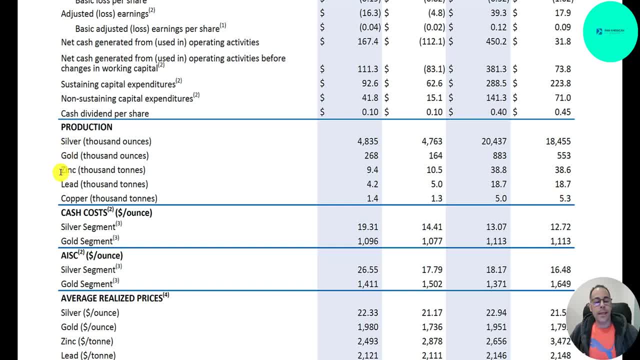 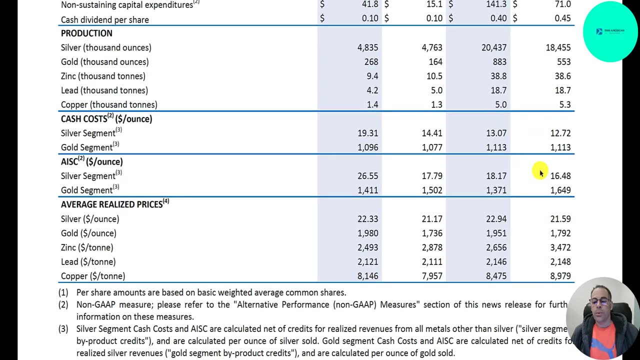 So these are their five main commodities: silver, gold, zinc, lead and copper. I'm really bullish on copper. I think that's going to go up the most because there's so much copper needed in the infrastructure for EVs and a lot of green energy. The all-in cost for silver went from 1,648 to 1,817 an ounce. The all-in cost for gold went down from 1,649 to 1,371.. By the end of 2023, gold was higher than the end of 2022.. The all-in costs went down. That's kind of interesting. I chose it right here: The average. 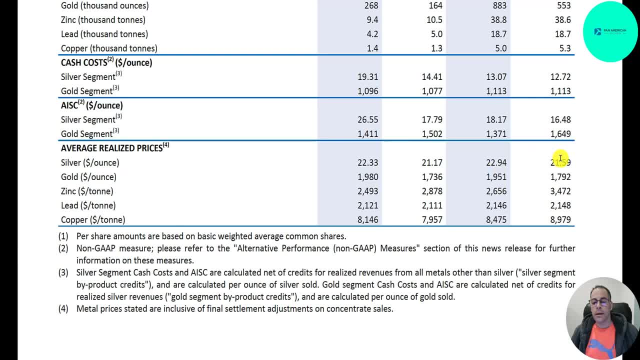 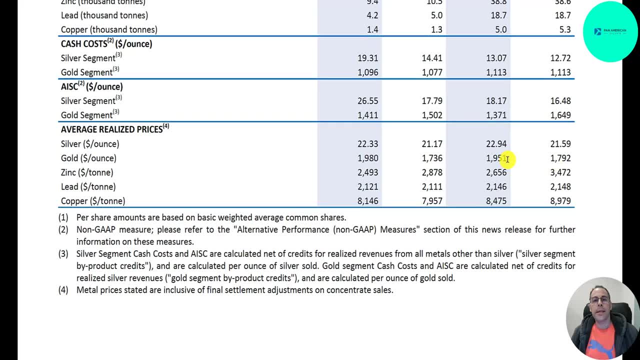 price for gold went from 1,800 to 1,950.. Silver went up a little bit. Zinc went down a lot. Lead was flat. Copper went down a little bit. These are the prices in the open market. Here's their income statement for the fourth quarter: Revenue of 670 million. 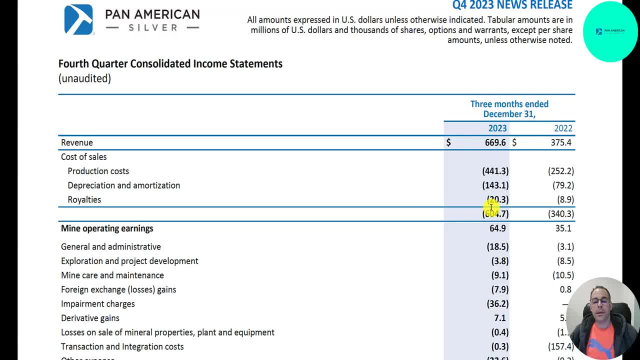 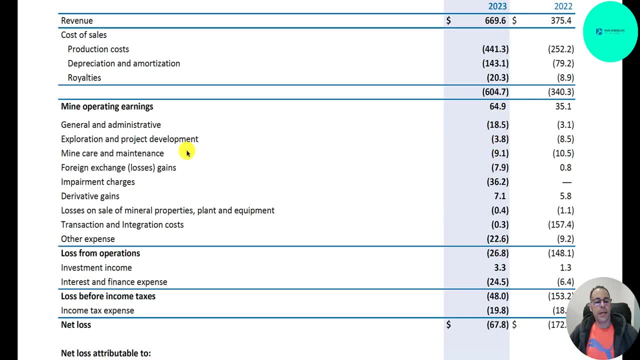 up from 375 million. Expenses of 600 million. Most of that is production costs- 440 million. Then you have lots of operating expenses: general and administrative exploration, mind care and maintenance Impairment. the biggest one, 36 million, That's when you write down the value of an asset on your. 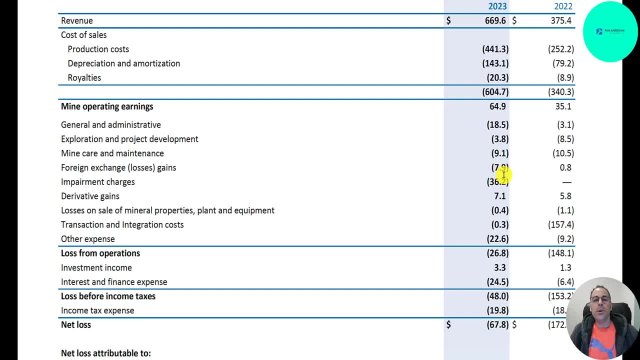 balance sheet and pass through a loss onto your income statement. When you depreciate an asset, it's normal wear and tear. Impairment is more extreme. You depreciate your car each year, say $2,000 a year for 15 years. But if your car gets totaled then you would impair it and write. 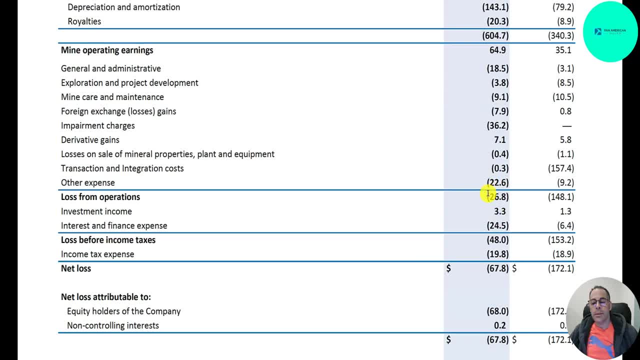 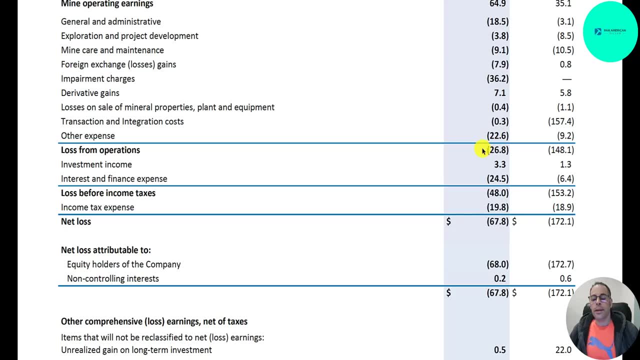 down the whole value of the car. They have an operating loss of 27 million compared to 148 million last year. They used to have an operating gain, like in 2020, 2021. Their expenses are getting pretty high. They need to fix that. 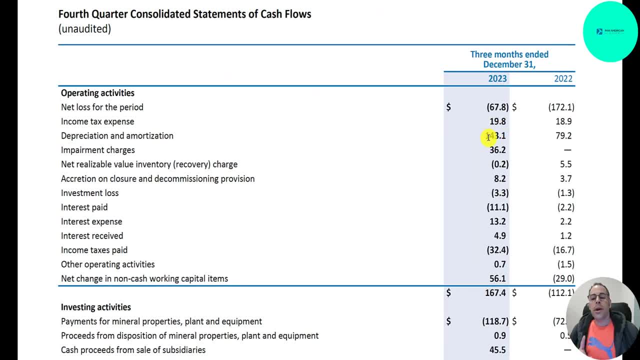 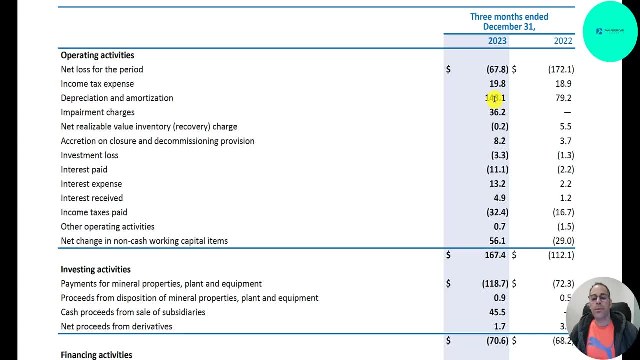 Here's their fourth quarter statement of cash flows. They do generate positive operating cash flow: positive 167 million. Maybe it's not that bad. They had a ton of depreciation: 140 million. That's a non-cash expense that brings down your net income, but we add it back here. 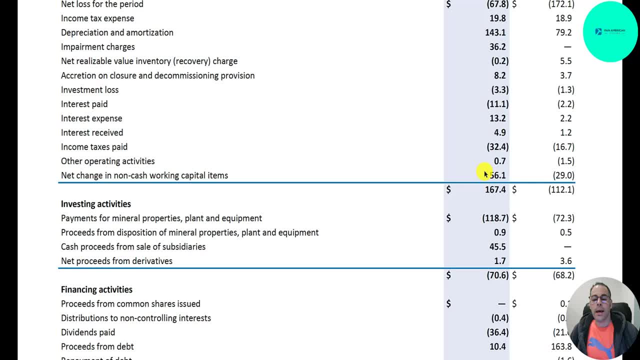 They also had a lot of depreciation, so they're getting a lot of depreciation. They're getting a lot of depreciation, so they're getting a lot of depreciation. so they're getting a $56 million cash inflow from working capital. So if they use accounts payable, that's a cash. 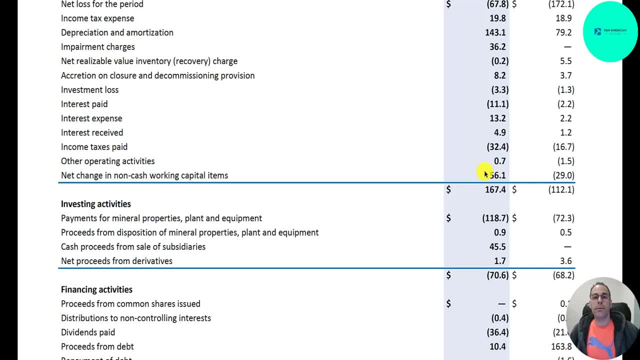 inflow, But when they pay back those accounts payable, it's a cash outflow. And when you buy inventory for your business, it's a cash outflow, But when you sell the inventory it's a cash inflow. It might sound a little confusing, but I did a video connecting the financial statements. 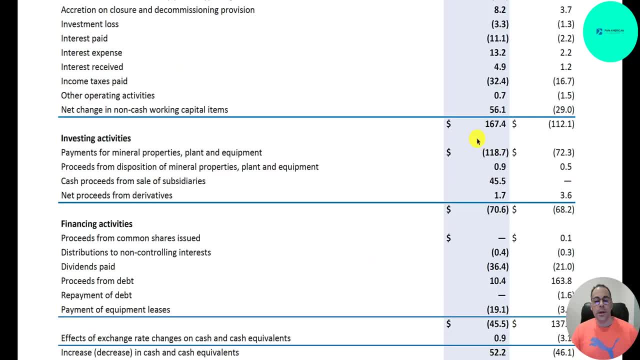 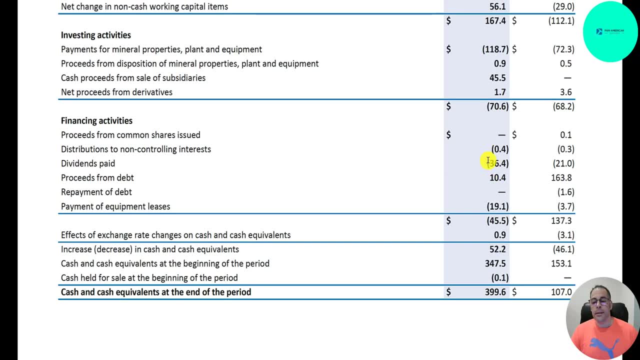 that explains this in more detail. They spent $119 million of PP&E- $70 million in the fourth quarter of last year. In their financing section they paid $36 million of dividends, about 50% higher than last year. They added $10 million of debt. Last year they added $160. 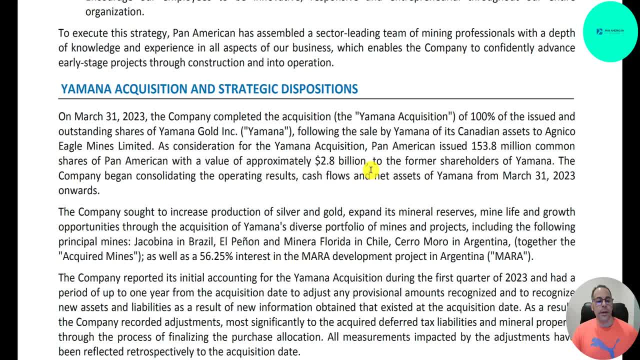 million. If you follow this company, I'm sure you're aware of the Yamana acquisition In March 2023, they acquired 100% of this company And that's why Pan American diluted their shareholders so much. They issued 154 million shares That was worth $2.8 billion to the former. 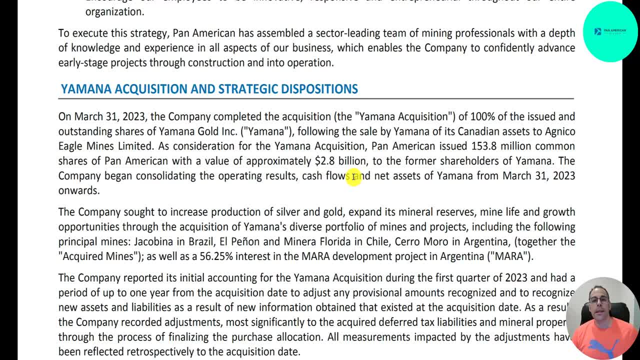 shareholders And that's why Pan American diluted their shareholders so much. That was worth $2.8 billion to the former shareholders And that's why Pan American diluted their shareholders so much. Since Pan American owns 100% of Yamana, they consolidate that company's operating results. 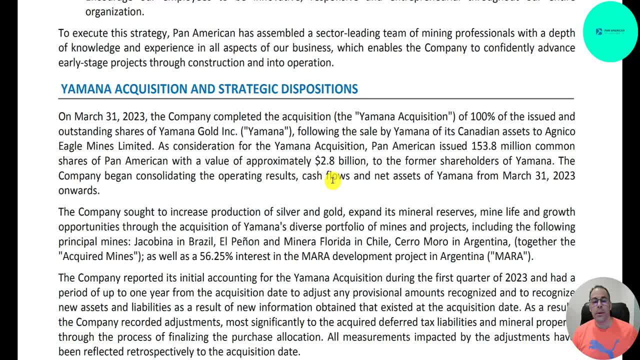 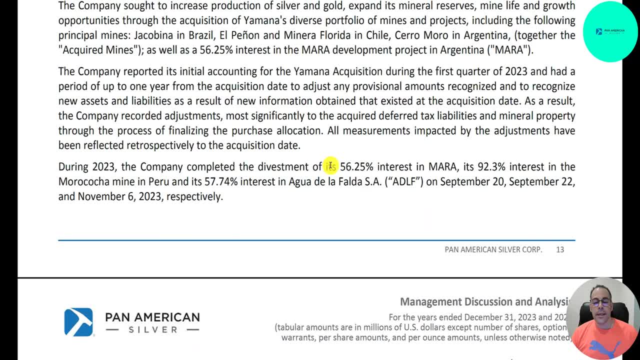 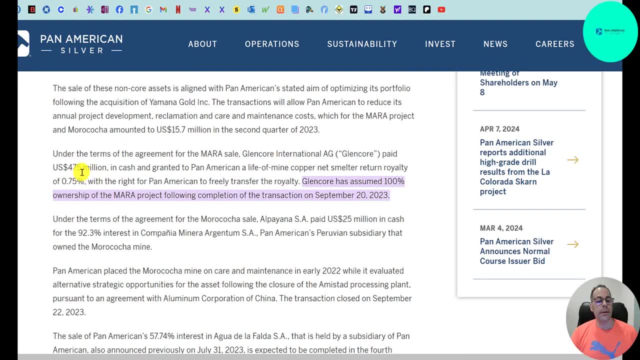 into theirs. So all of Yamana's revenue, all Yamana's expenses, all their debt are part of this company's financials. They also divested Mara to Glencore, And it talks about it in this article. Glencore paid $475 million to Pan American, So now Glencore has assumed 100%. ownership, And that's why Pan American diluted their shareholders, And that's why Pan American diluted their shareholders, And that's why Pan American diluted their shareholders And that's why Glencore paid $475 million to Pan American. So now Glencore paid $475 million to Pan American. 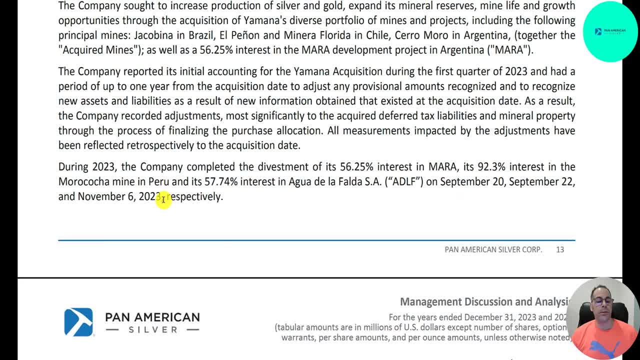 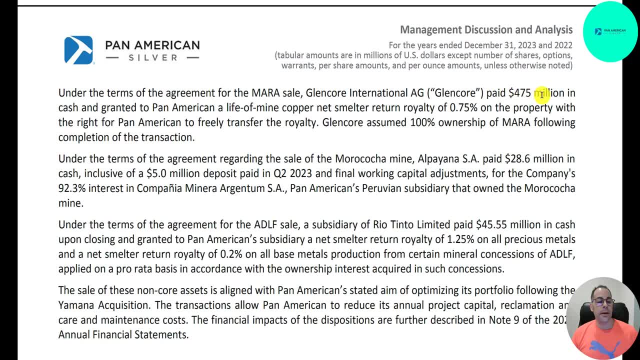 They also divested other assets: a 92% interest of a mine in Peru and some other things. It's right here on the next page, if I just waited and looked. Glencore paid $475 million in cash to Pan American For the Peruvian mine. Pan American received $29 million in cash. 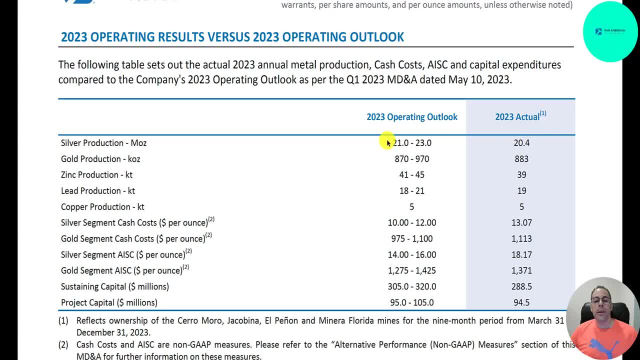 They actually produced 20 million ounces of silver, which is below their outlook. They forecasted $21 to $23 million. They did hit their goal target. They actually produced $880,000.. The forecast is the $870,000 to $970,000, so the lower end of the forecast. 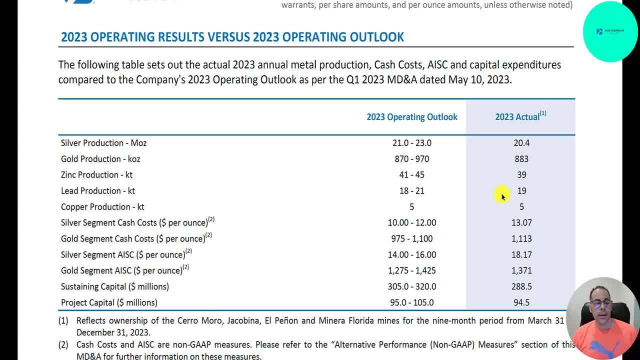 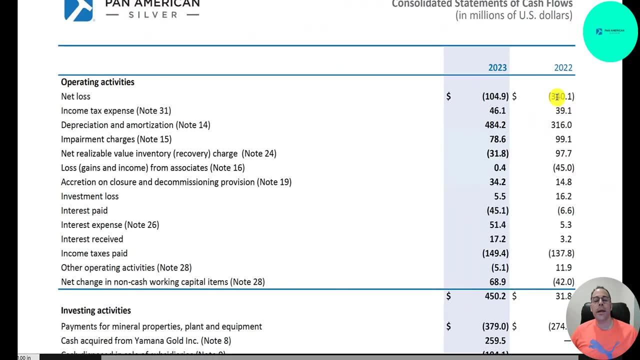 They fell short on zinc. They hit their lead target And they hit their copper target. Their all-in cost for silver are higher: $1817.. The target was $14 to $16.. Gold: they were on target: $1371,, which is between their forecasts. Here's their statement of cash flows for all of 2023.. 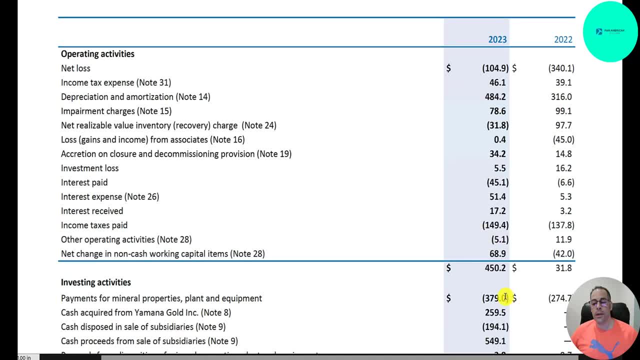 Earlier. we just looked at the quarter. So for all of 2023 it looks pretty good, Operating cash flow of $450 million. That's up a lot from last year of $32 million. Even though they had a net loss of $100 million, they still generated $450 million of cash flow. 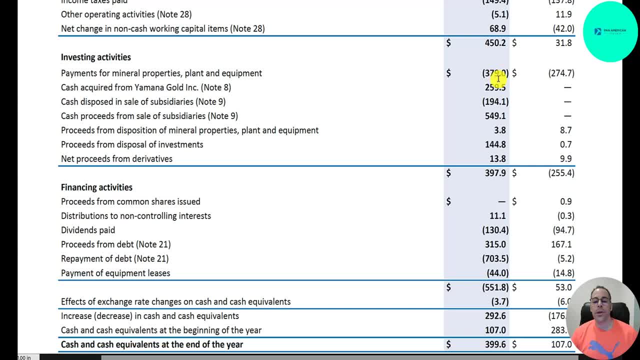 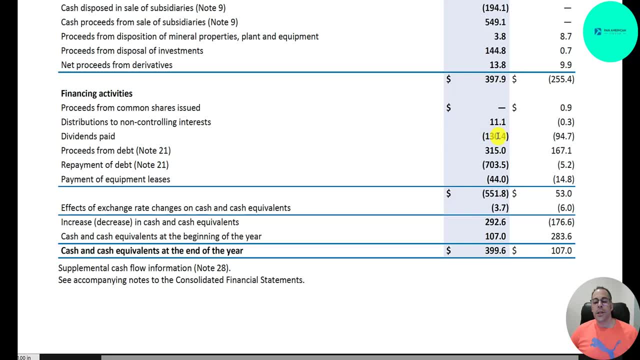 In the investing section you can see all the acquisitions: $379 million of PP&E, A cash inflow of $259 million from Yamana Gold. In the financing section they paid $130 million of dividends- $95 million last year. They added $315 million of debt paid down $700. 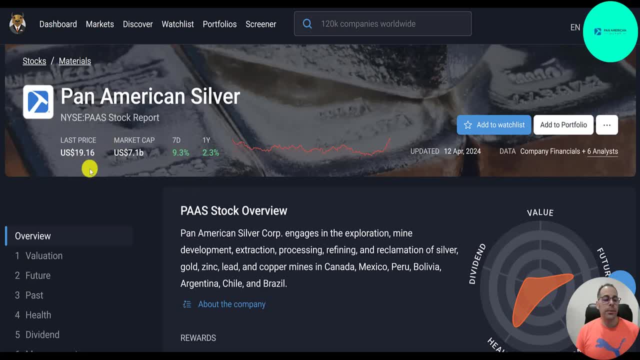 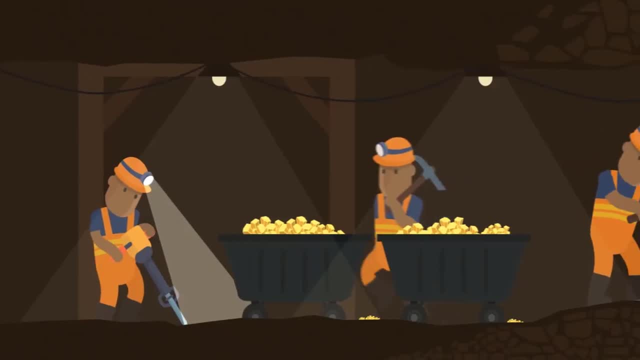 million. Let's take a look at the stock on Simply Wall Street. It's last price: $19, $7.1 billion. market cap: Up 9% in the past week, Up 2% in the past year. Let's see what they say about the company. 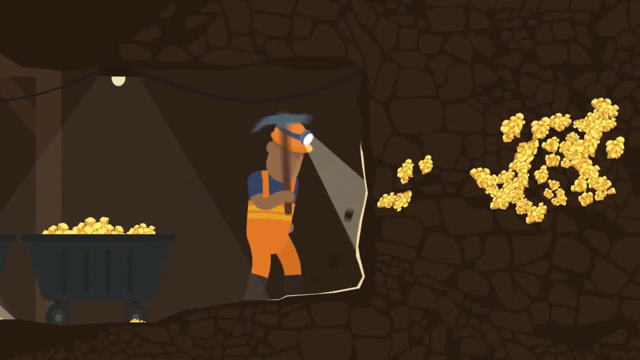 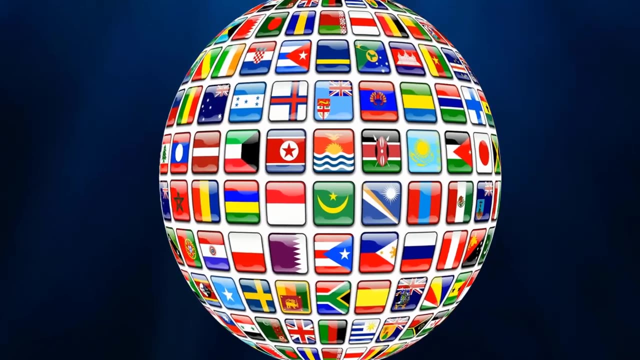 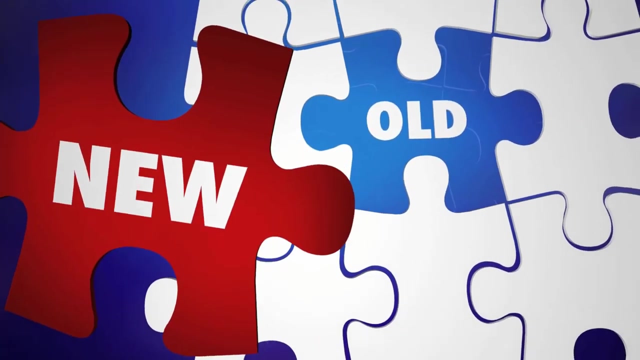 Pan American engages in exploration, mine development, extraction, processing, refining and reclamation of silver, gold, zinc, lead and copper mines in Canada, Mexico, Peru, Bolivia, Argentina, Chile and Brazil. They were formerly known as Pan American Minerals Corp And. 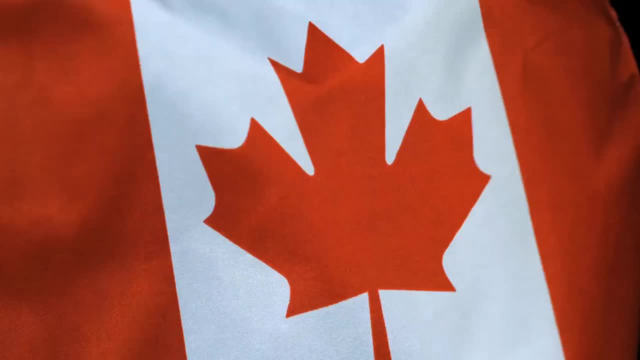 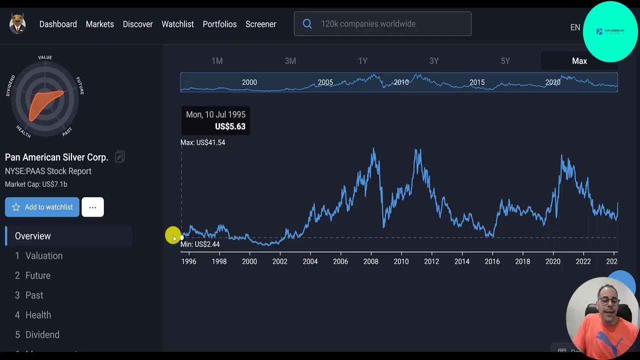 they changed their name to Pan American Silver in 1995.. Incorporated in 1979, headquartered in Vancouver, British Columbia, Canada, It looks like they started trading in 1995 at $563 a share. Its lowest point was in 2001,, between $2 and $3. 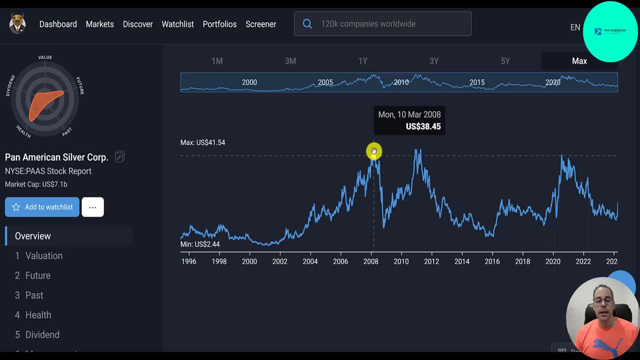 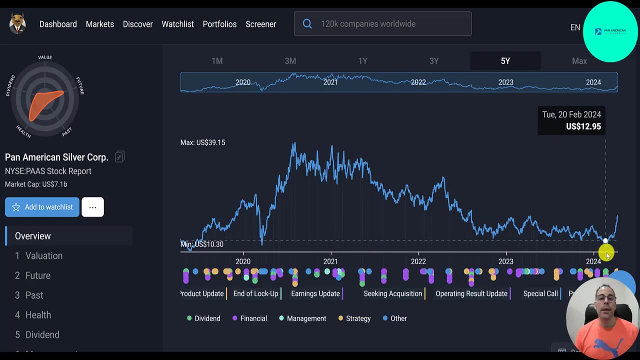 a share And you can see how volatile the stock is. It ran up past $40 in 2008,, then down to $10 at the end of 2008,, back up to $40 in 2011.. In 2011, it was down to $6 in 2015,, back up to $40 in 2020.. In the beginning of this year, 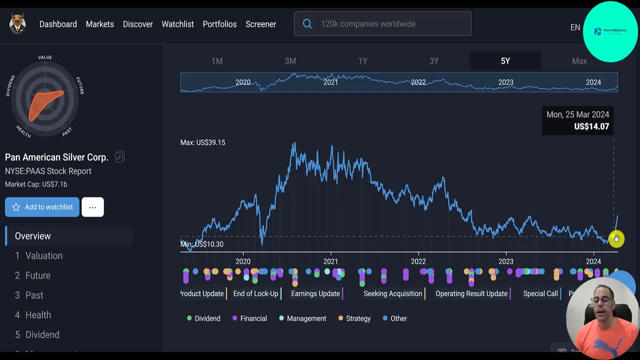 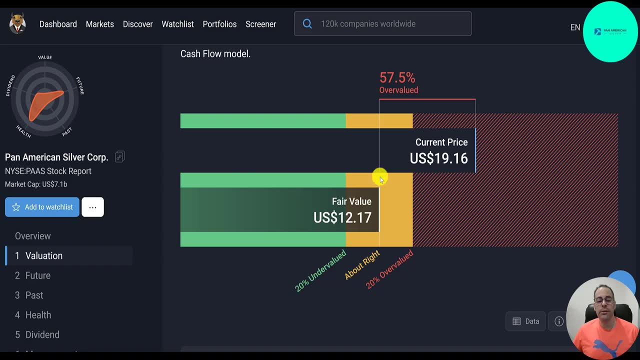 it was as low as $13 a share, But it is coming back up. If the price of silver or gold goes up, this stock should go up Simply. Wall Street's valuation is $12.. They say the stock is overvalued. 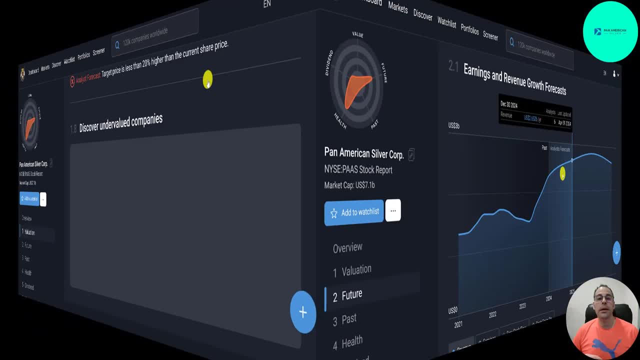 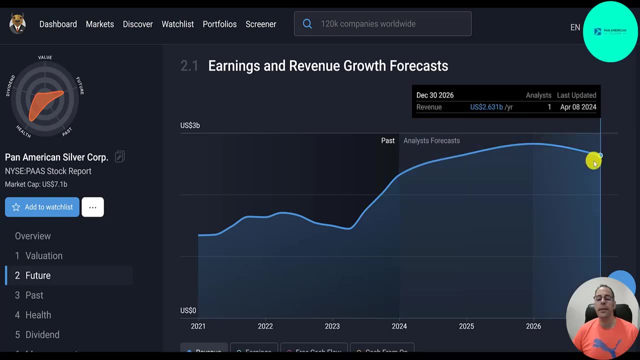 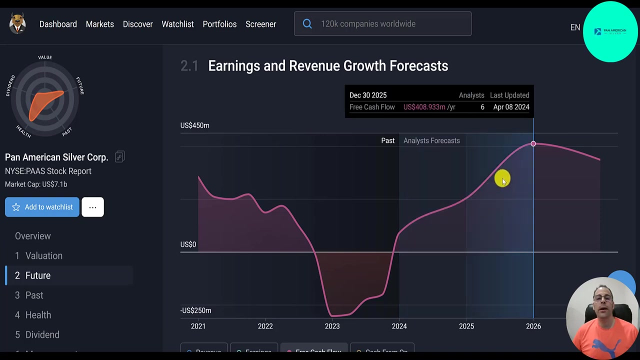 Two analysts priced this stock at $23.. The revenue forecast for 2024 is $2.65 billion- $2.65 billion- $2.8 billion, $2.26 billion, back down to $2.6 billion, And the free cash flow forecast for 2024 is $200 million- $2.25 billion- $4.00 billion. 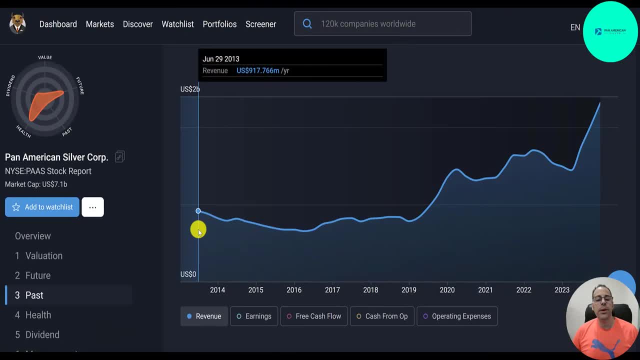 $2.26 billion down to $348 million. You can see that revenue has come up a lot since 2013.. It was a little over $900 million And then it was pretty flat for the next 5 or 6 years. 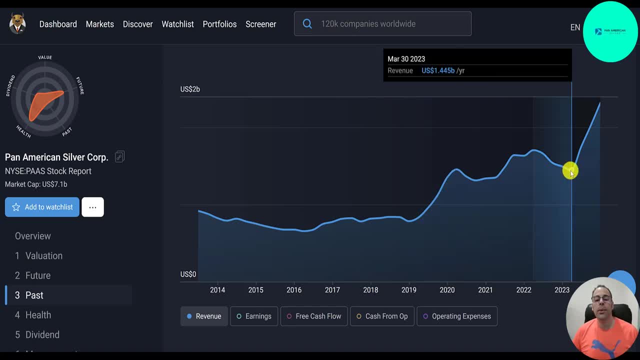 Then it jumped up to $1.5 billion in 2020.. Still around $1.5 billion for the 12 months ending 3-31-2023.. Then, with their acquisitions- the Yamana acquisition- it has come up to $2.3 billion.